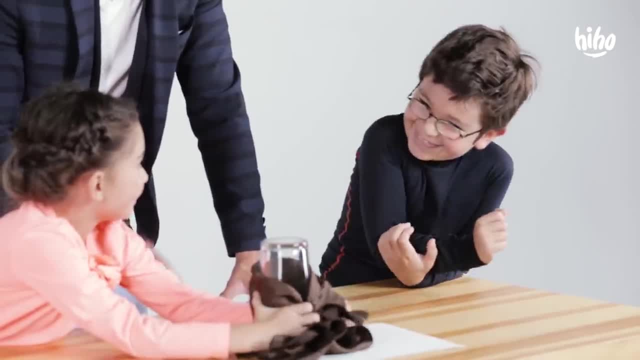 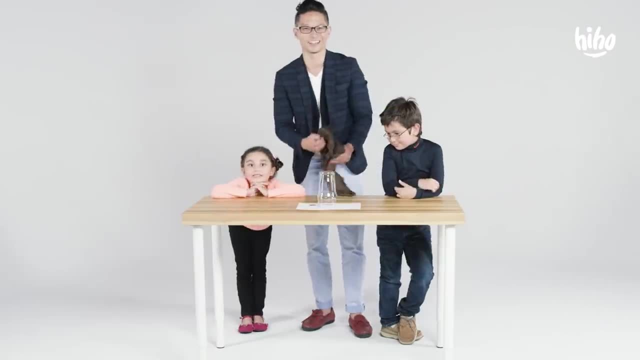 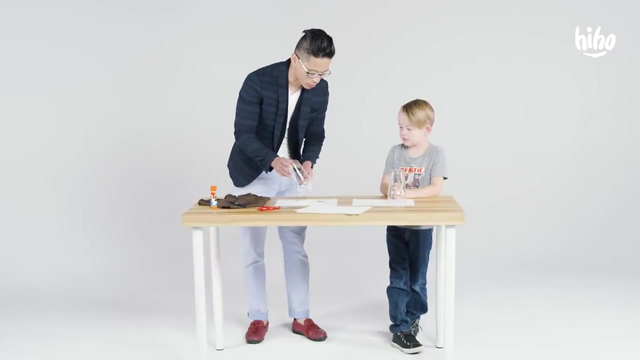 what the here? how did you? what did you see it? look, let's look, it's gone. i think you did that. that was good. she did it and you didn't. she didn't even see it. you see, this glass is a tricky glass because on the bottom it has a piece of taper. 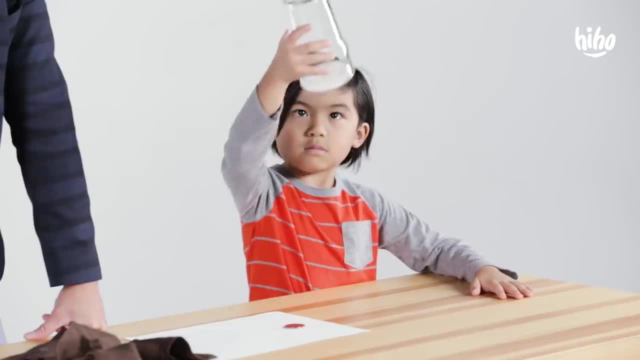 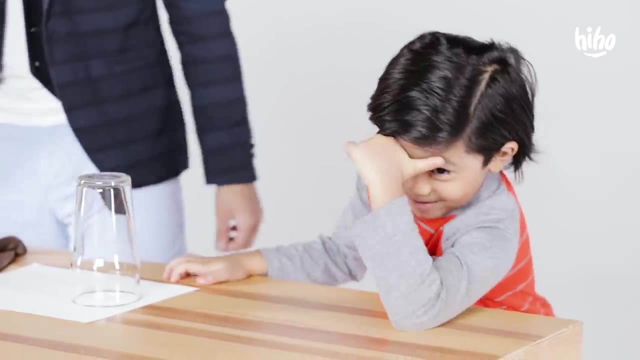 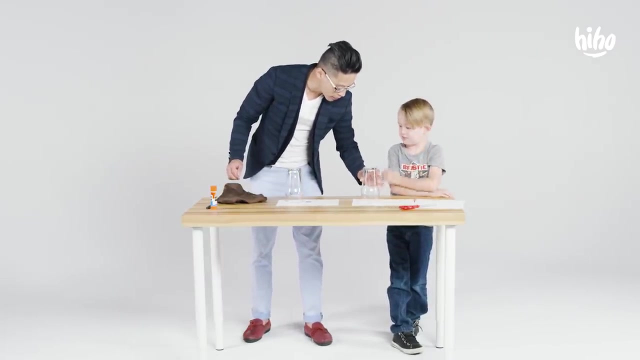 right, not, not that way. you gotta. you're gonna make one, i'm gonna teach you how to make one. yeah, hey, um, Wow, okay, i'm gonna teach how to make a glass. okay, ready, all right, so put the cup over the piece of paper, like that. 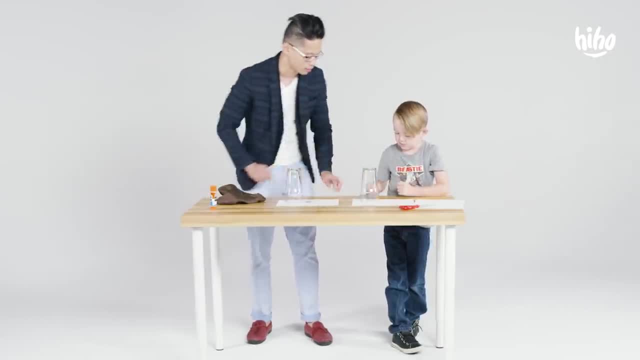 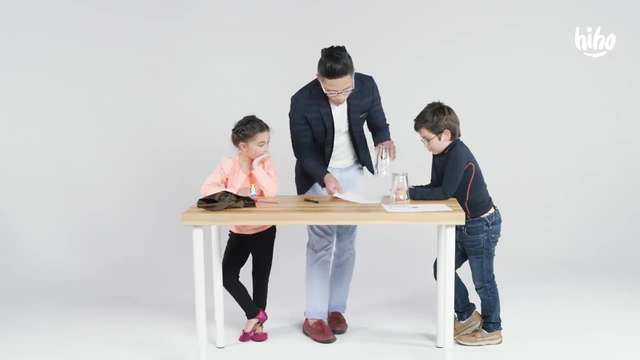 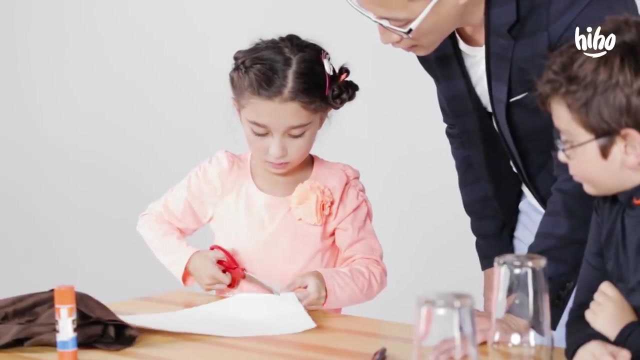 all right now, once you go ahead and trace around the mouth with the pen, go for it. so far, so good. now that you have this right here, Helena, i want you to very, very carefully go ahead and cut this out very, very careful- like even more careful than that. i want you to glue this onto the cup. 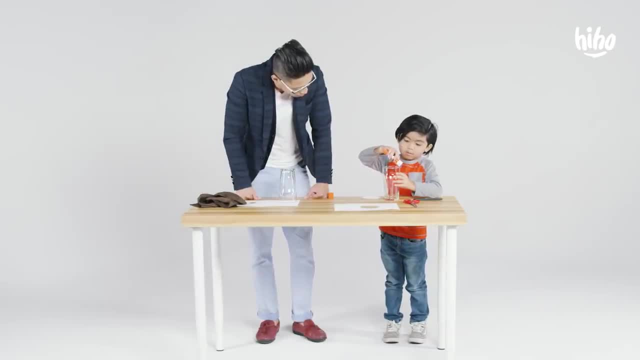 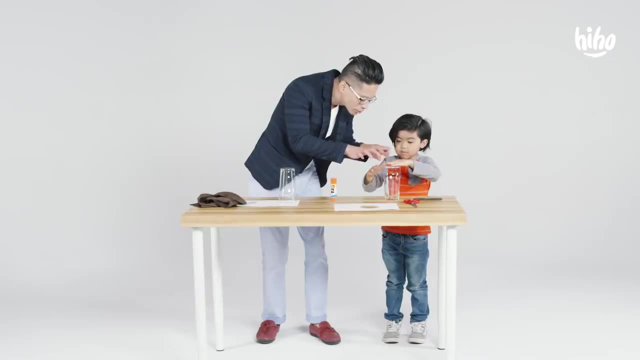 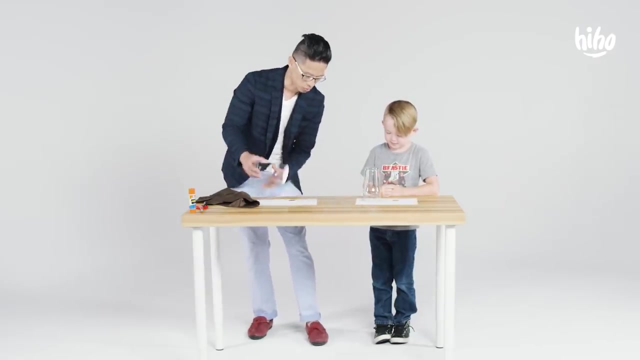 okay, all right. yes, this is good. okay, so make sure you're secure, run your finger around, all right. so you want to begin the trick like this: you got a piece of paper and you got the mouth down like that: don't, don't do this, this is big. 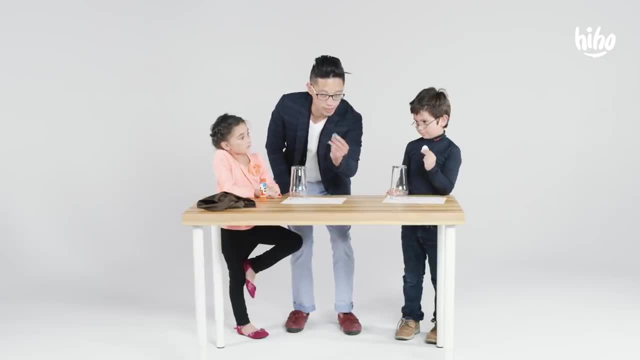 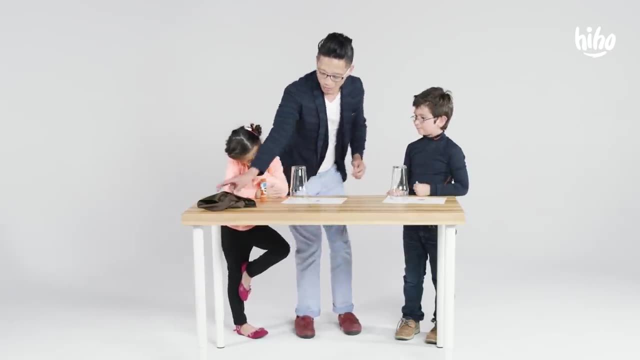 secret. you got it. good, yeah, hold a coin like that and say I'll make the coin disappear. all right, I put this on the paper like that. good, I'm gonna give you a piece of cloth. okay, then can you cover the cup with this piece of cloth? 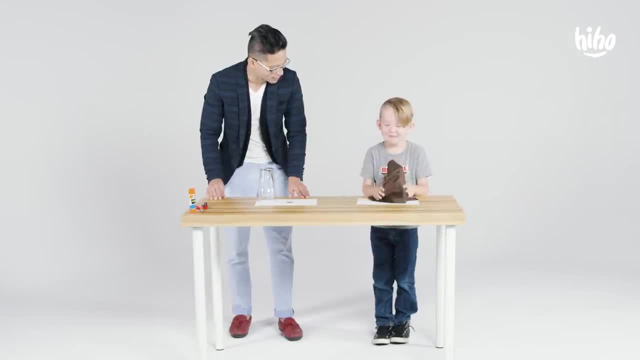 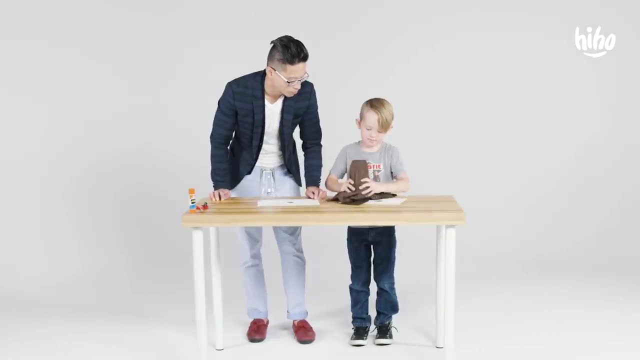 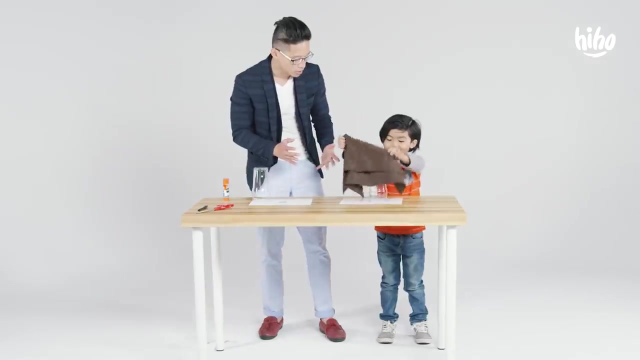 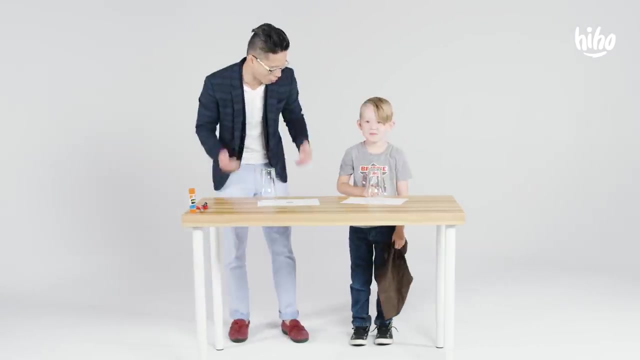 go for it, okay. and you put it: is that over the coin? oh, you gotta make sure someone's going. so do it again, do it again, do it again, okay, no, okay. then say abacadabra, and what? where is it Desmond? where is it Desmond? where is it Desmond? let's bring it back, okay. so cover the.